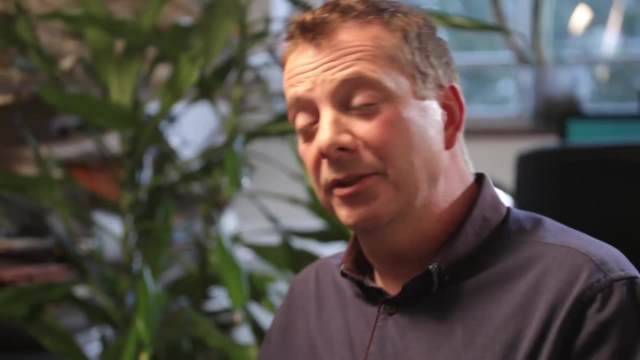 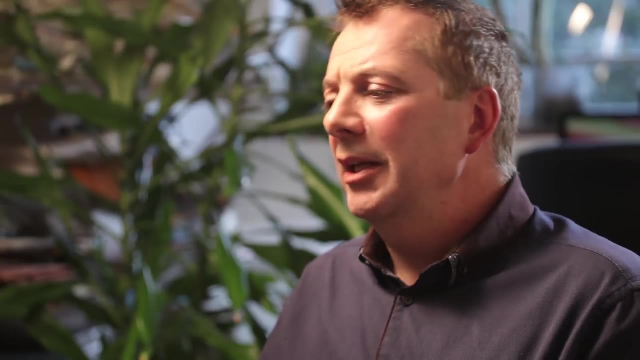 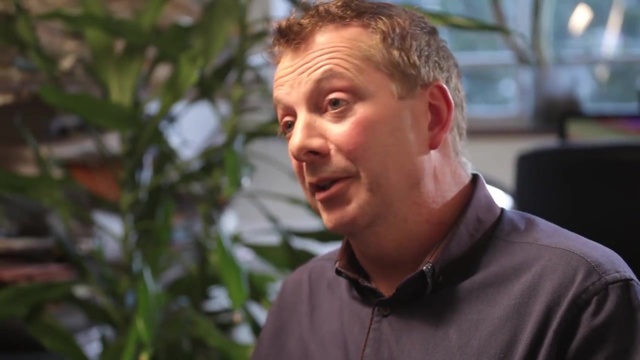 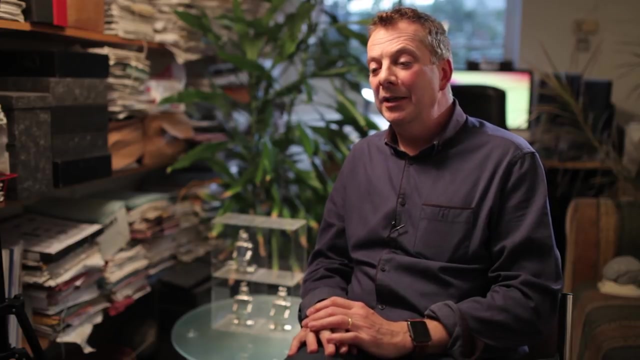 of economic resources they have, but also aspects of social hierarchy, of prestige, of power. So typically in studies we might measure it by looking at the level of the parent's education or we might look at the family income. One of the most striking features of socio-economic status on children's development is that by 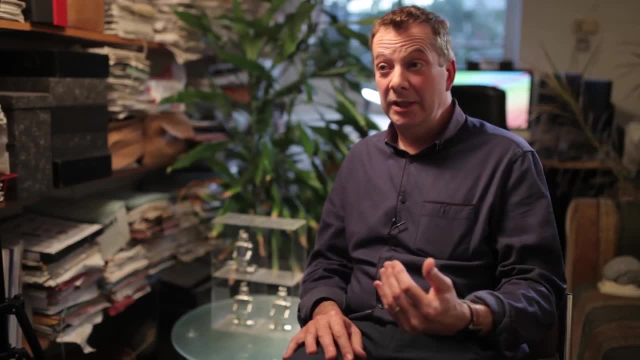 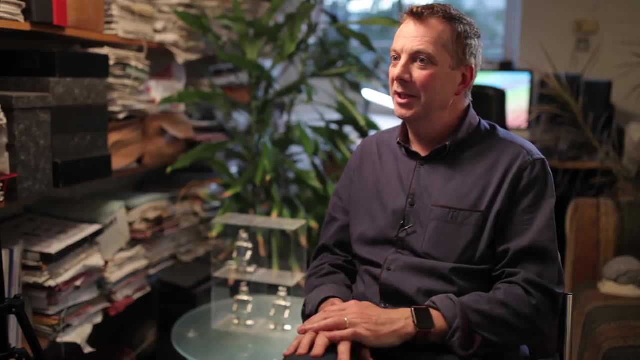 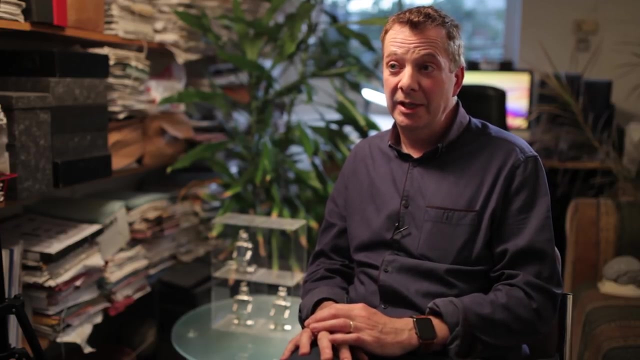 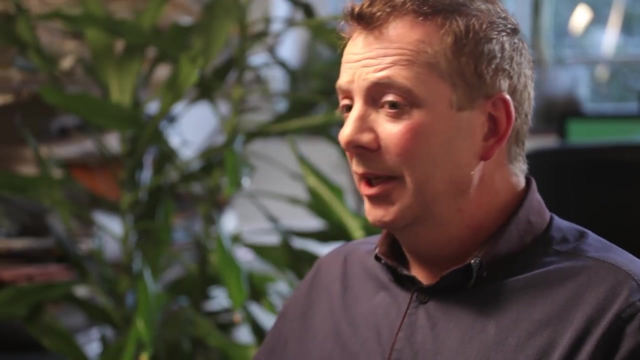 the time children start school, you can already see big gaps in their behaviors and their cognitive abilities, say the vocabulary size of children according to the socio-economic status, Or I'll call it SES, the SES of the families they come from. And once children start school- 3,, 4,, 5 years of age- those gaps they don't narrow. They 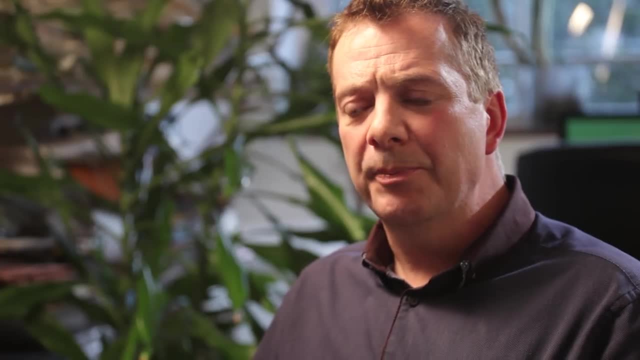 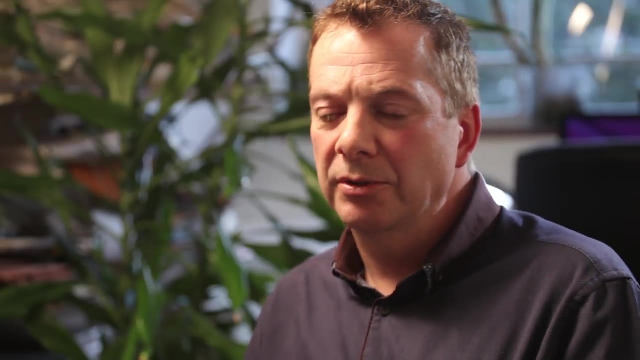 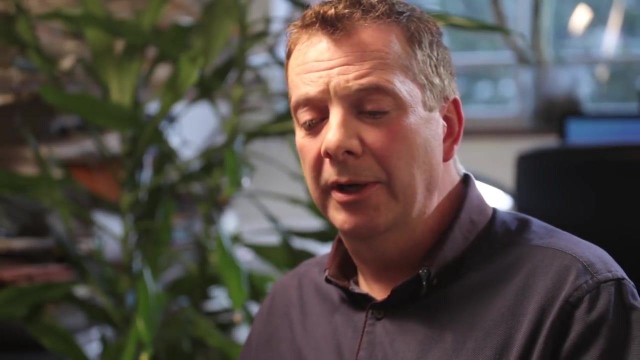 often persist throughout the school years. So there's a big concern there. What are these influences of socio-economic status, How are they impacting on children And what can we do about that to try and close the gaps caused by the differences in family background? 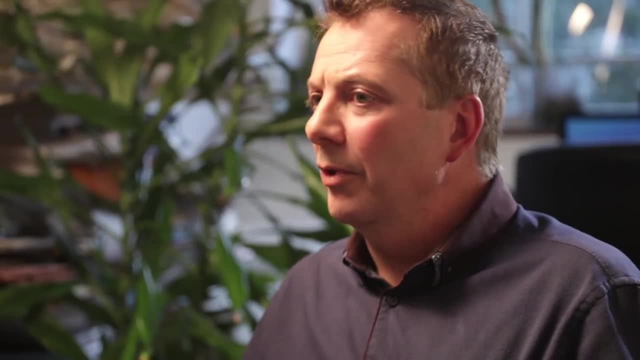 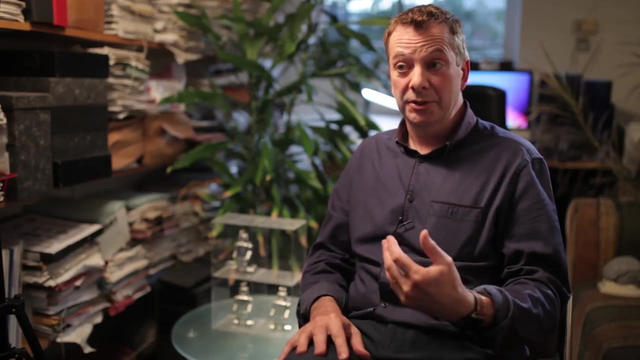 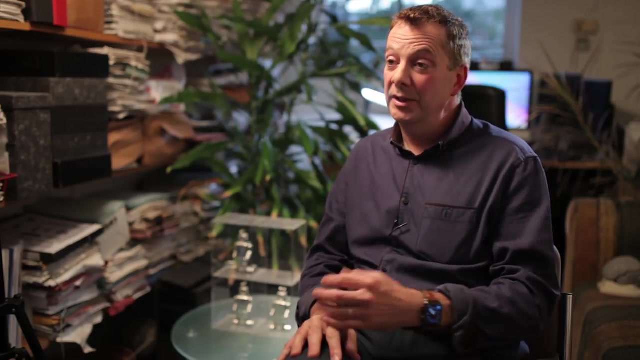 So that is the goal of cognitive neuroscience: to understand mechanisms. If we understand causes, that enables us to try and intervene and to figure out the easiest way to ameliorate, to reduce the consequences on children's development of these differences in family background. 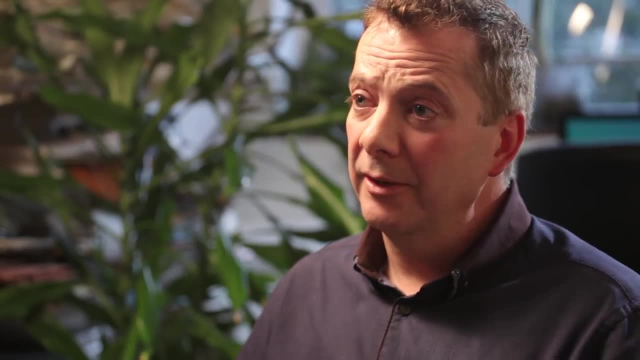 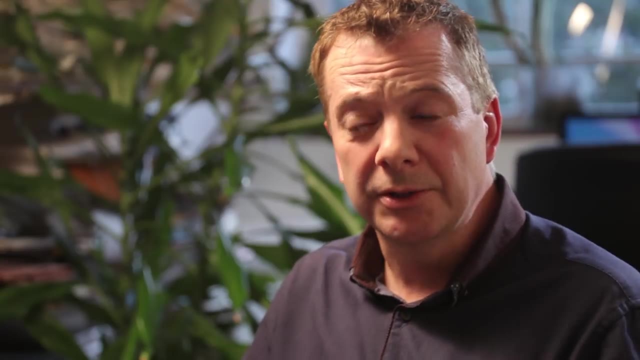 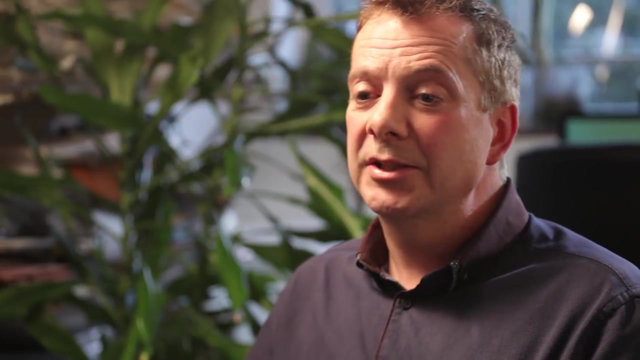 So if you look at behavior, what's interesting about the effects of SES on behavior is that they're uneven across different abilities. In fact, that's one of the puzzles. For instance, there was one study by Daniel Hankman and Martha Farah suggested that perhaps a third of the variation in children's vocabulary size their 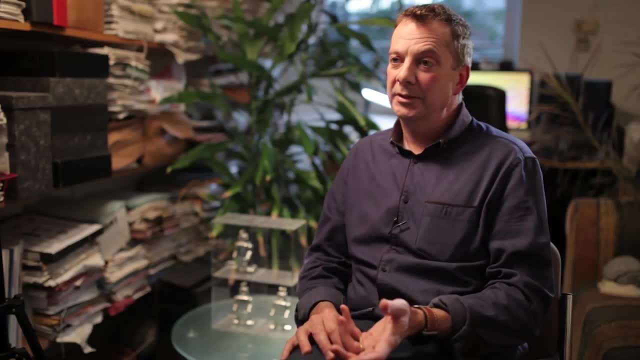 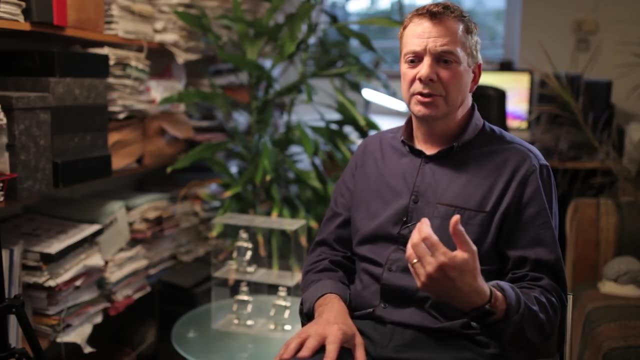 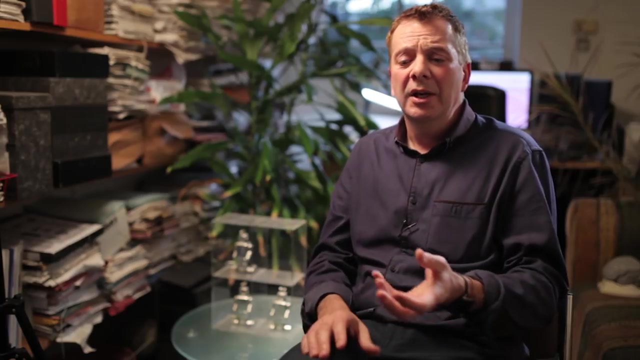 language development can be explained by socio-economic status. That's a large amount of variability. If you look at areas of behavioral regulation- whether they can control or inhibit their cognitive functions- Executive functions- About 6% of the variation is explained by socio-economic status. 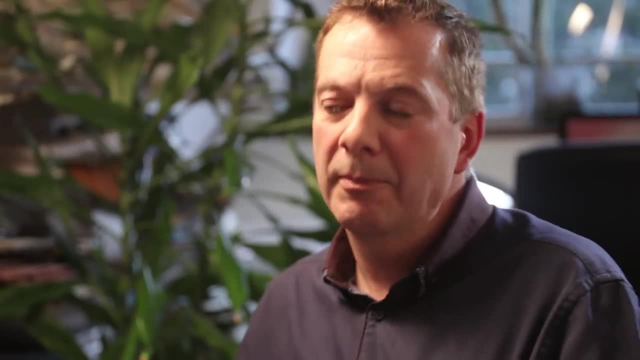 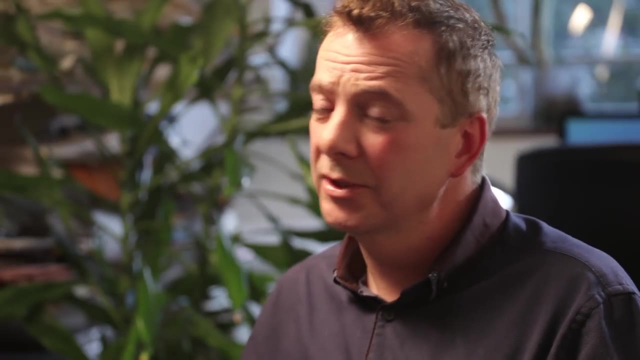 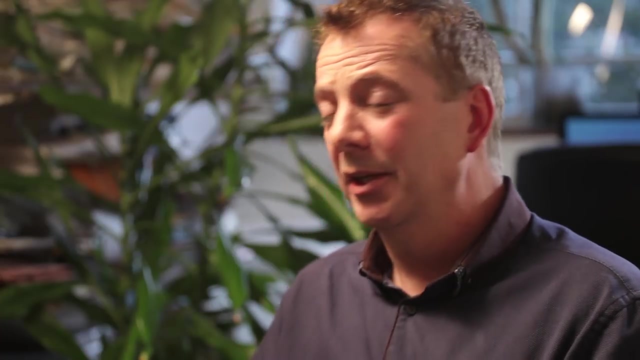 A similar amount is explained in the variation of their working memory ability, what they can keep in mind. But then you look at something like their visuospatial skills, working in space, remembering spatial configurations. There's not much influence of socio-economic status on that aspect. 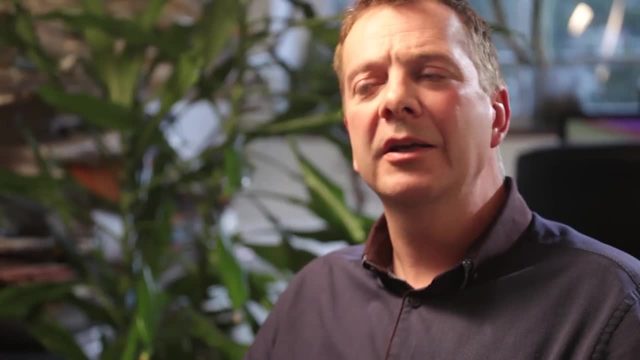 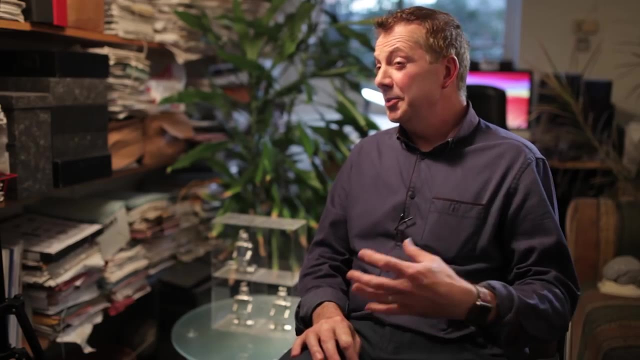 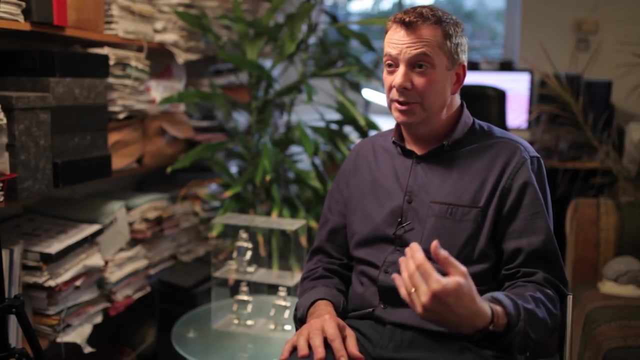 So why is it that socio-economic status would have that uneven kind of influence across the development of different kinds of skills in children? Ultimately, we expect socio-economic status to have a biological influence at some level, And so one of the places we want to start is to investigate what effects socio-economic 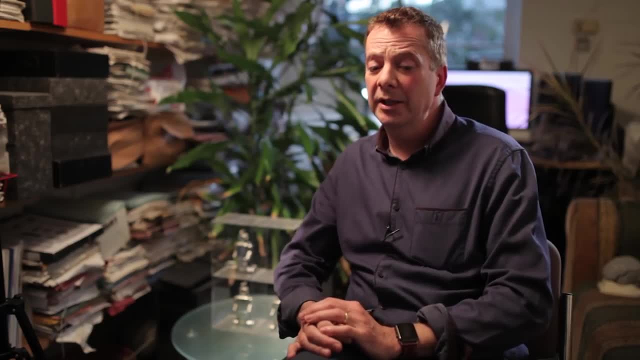 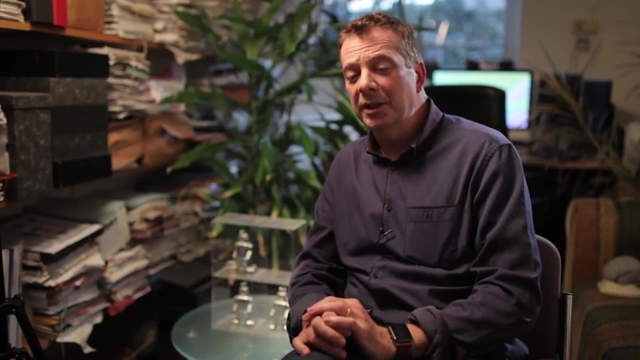 status may have on the brain. So let me give you an example of a study which was a large study looking at- I think it was- 1,000 children in the US And this was a study. It was led by Kimberley Noble. 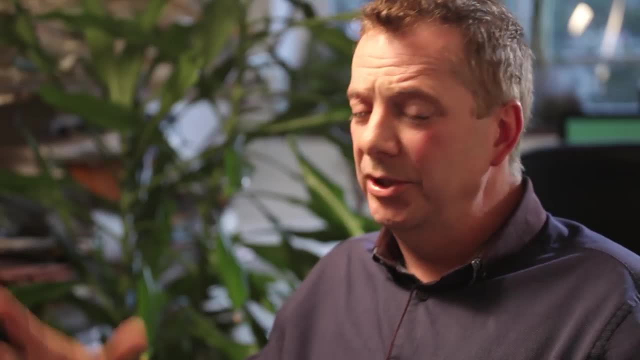 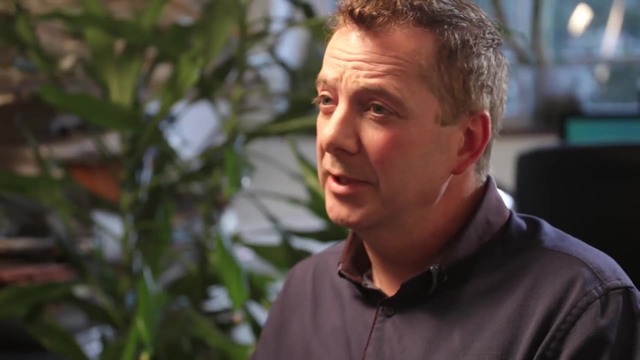 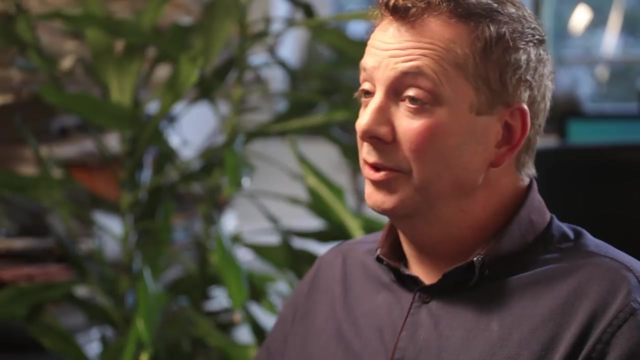 What they did was to scan the brain structure of these 1,000 children and look in detail at the surface area of the cortex, the thickness of the cortex, and see whether they could detect the impact of the family's socio-economic status on children's brain structure. 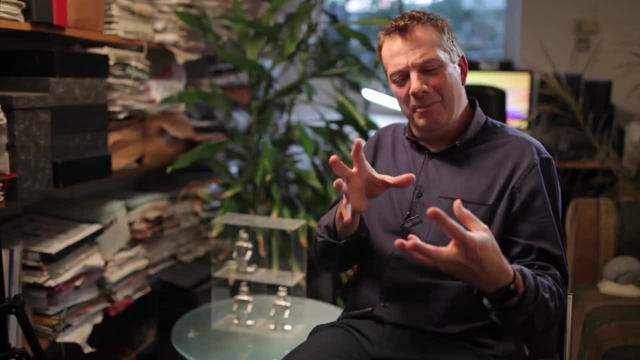 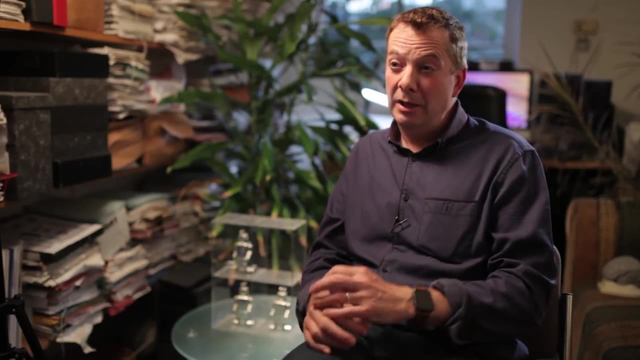 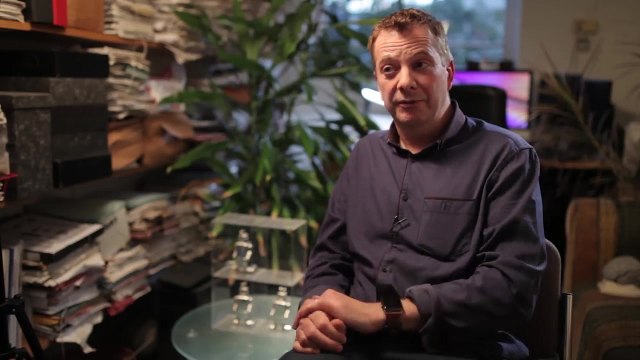 Now, this is a very kind of gross measure, looking at just the amount of white matter and gray matter, And the effects are quite small. The researchers needed a large sample in order to detect these differences, But ultimately they did show variations, particularly in cortical surface area, according. 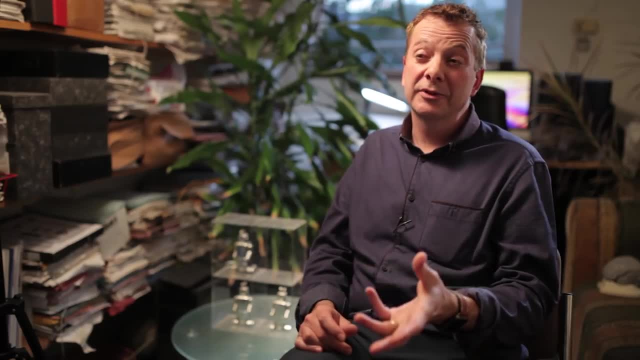 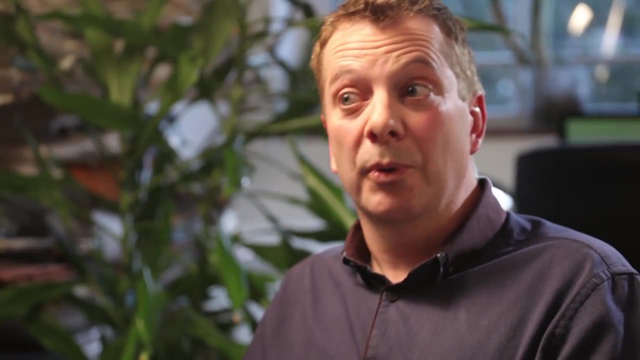 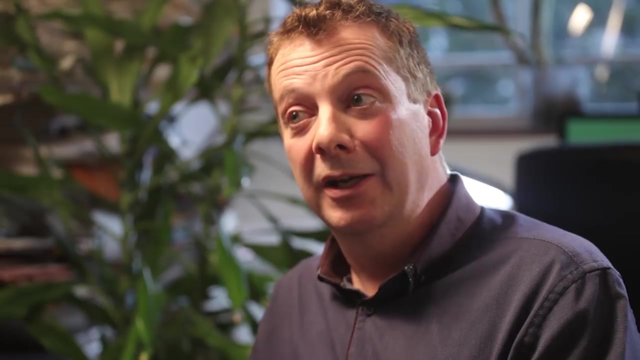 to socio-economic status. Interestingly, the differences they found were in temporal regions and in frontal regions of the brain, And that fits with what we see in behavior, that temporal regions of the brain are involved in language processing. The frontal regions of the brain are involved in executive function. 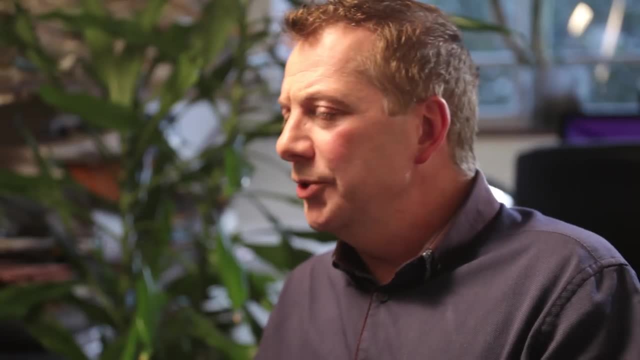 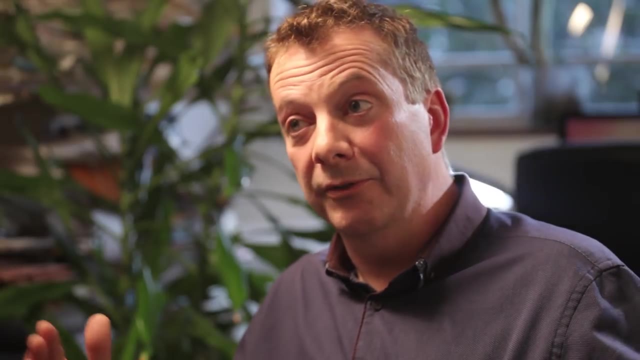 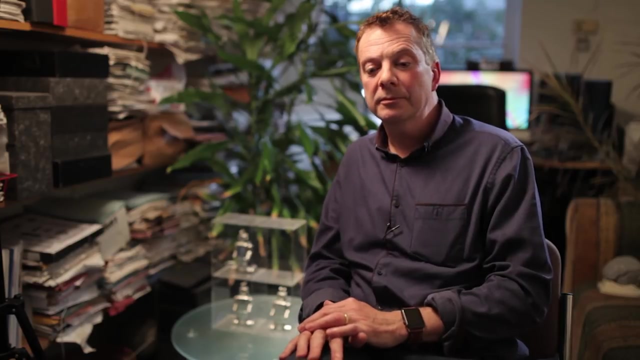 So it fits with what we're seeing in behavior. It's also possible that those parts of the brain have the longest developmental trajectory, And maybe this long period of development for temporal and frontal regions gives the most opportunity for the environment to influence their development. 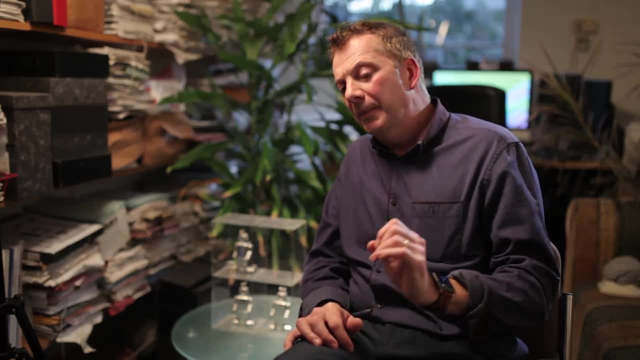 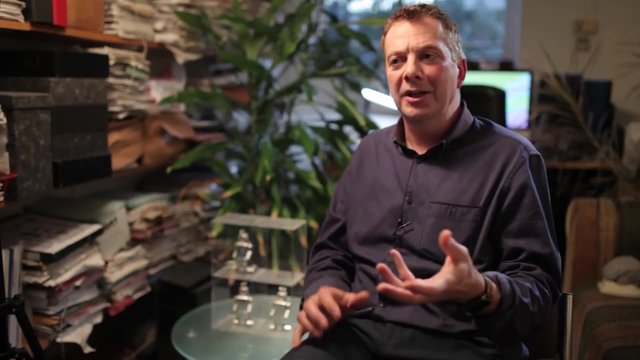 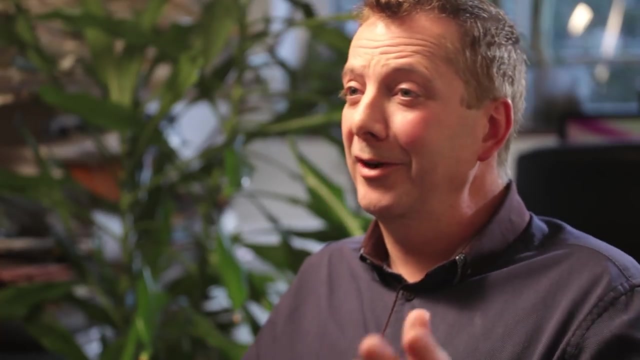 A couple of other things you might say about that. The effects were really quite small. There were only one or two percent of the variation in brain structure was being explained by socio-economic status, Even though, as I said, about a third of the variation in language development was predicted. 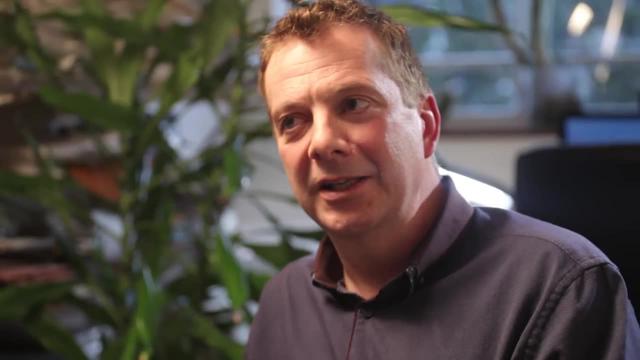 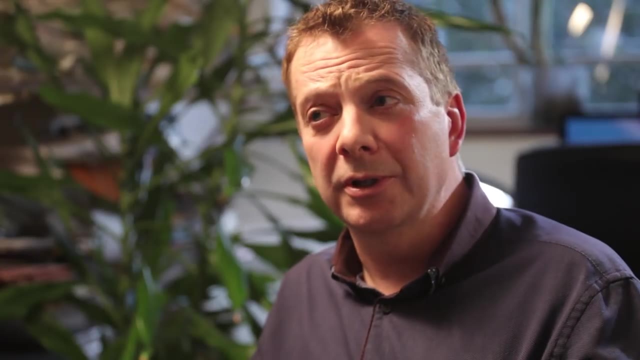 by that same error. So it's more obvious in behavior than it is in these subtle measures of brain structure. That's just looking at structure, but you can also look at the function of the brain. So one of the things we can look at is the function of the brain. 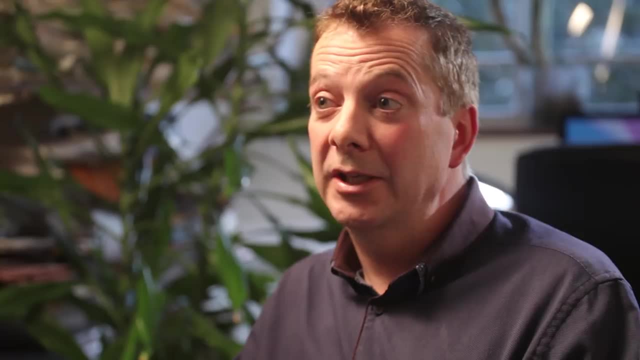 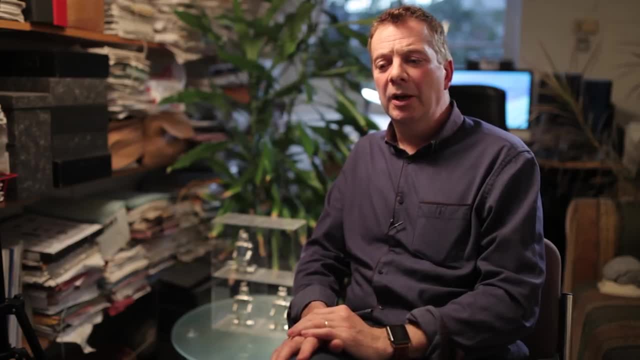 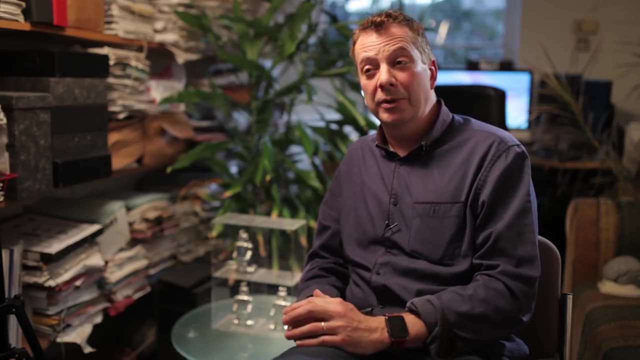 it at the scalp using electrodes. These are very small voltages and what you can do is to see changes in those voltages as children carry out tasks. So there was a study carried out by Courtney Stevens and Helen Neville where they played children different sounds. 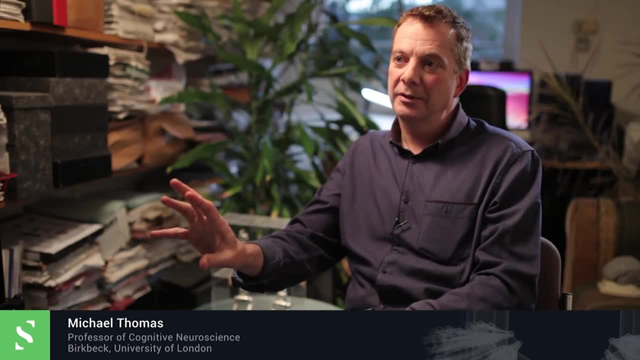 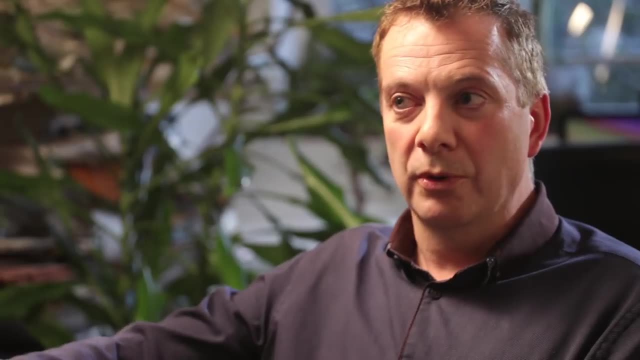 And they were only supposed to pay attention to one of the sounds and ignore the other sound And children from a low socio-economic status back. their brains were less able to ignore, to screen out the information that they were not supposed to pay attention to. 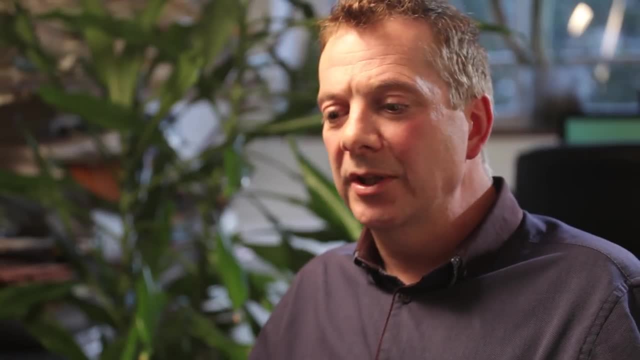 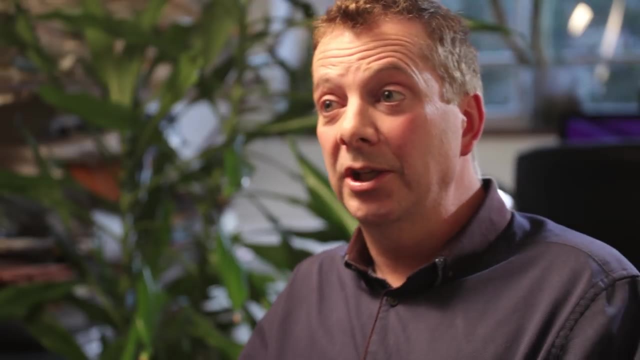 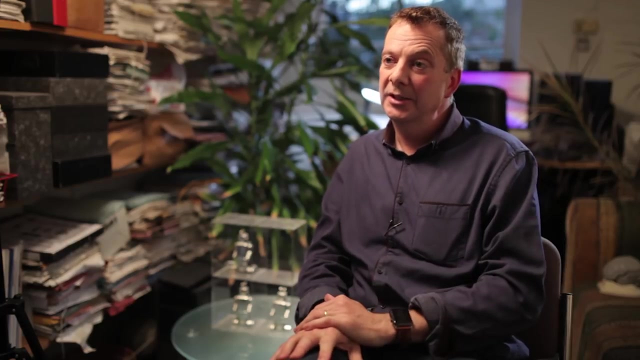 So the suggestion there was that there was a problem in selective attention in those children. So both evidence on brain structure and evidence on brain function, that socioeconomic status is having an effect at a biological level. Well, we have to think about how that's going to work. 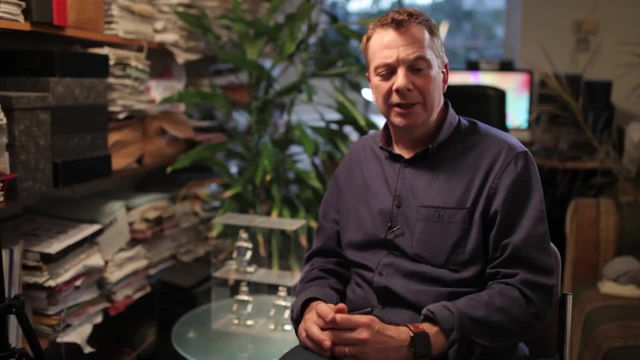 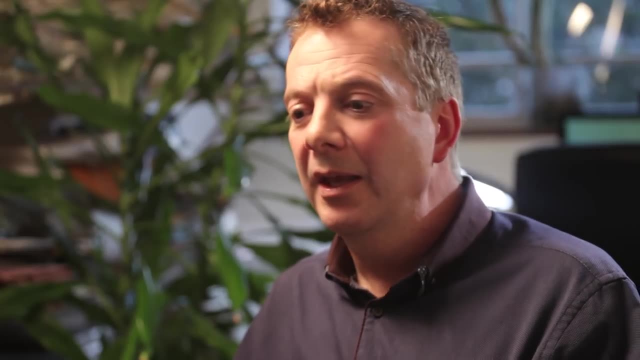 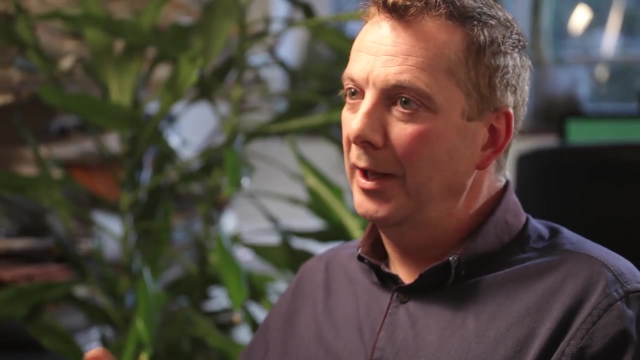 What is the actual pathway between which you have these things that you measure in the environment and these effects on brain structure and brain function? Here, as scientists, we run into a bit of a problem. So the problem is, we like to detect correlations and they suggest causal pathways. 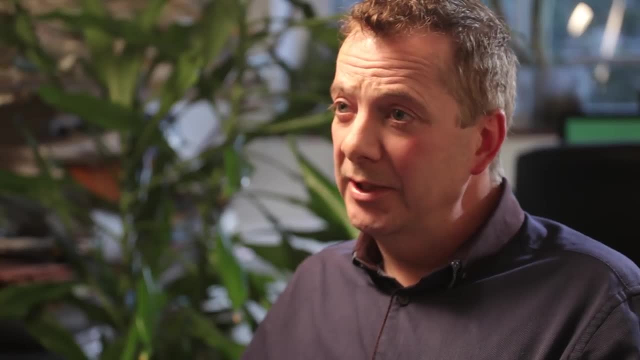 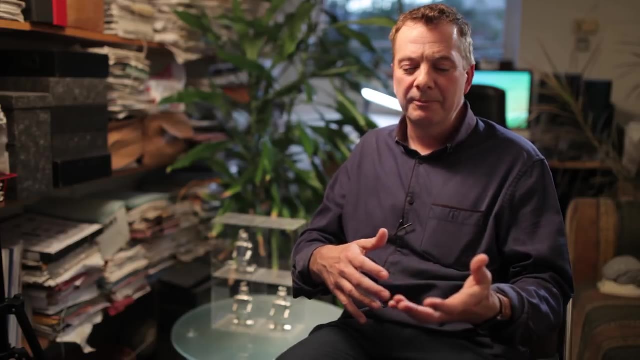 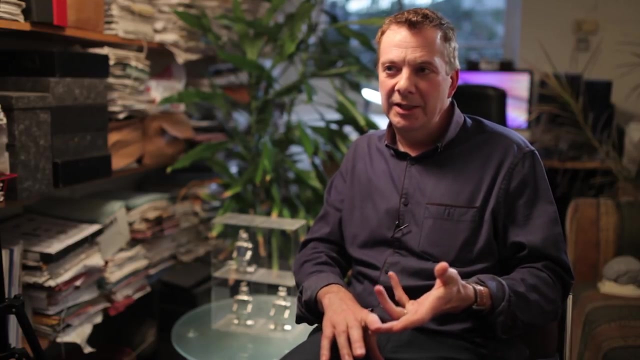 But what we have with socioeconomic status is that we don't have a causal pathway. We have a kind of a mashing together of lots of correlated factors in the environment. The family that has fewer resources, that they're poorer. The parents may be less educated. 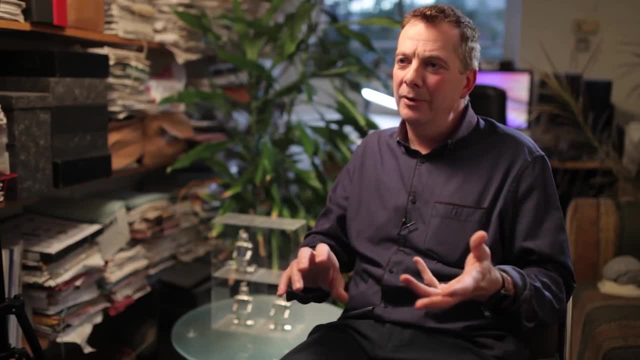 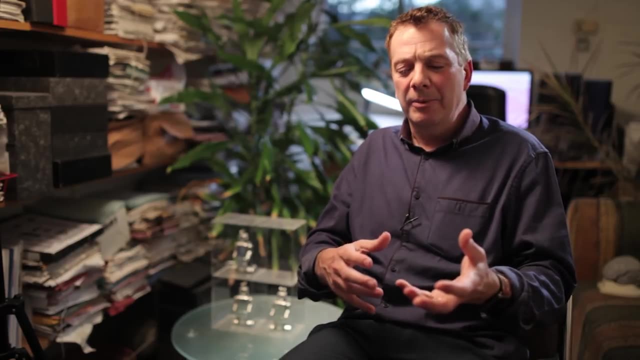 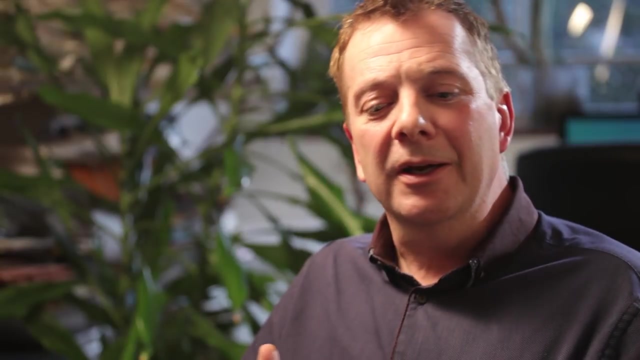 The household may be in a poorer neighborhood. It may be a less structured household. There may be fewer resources, fewer books, fewer toys And maybe the parents interact with the children differently. They're more stressed. They have less quality time With the children. the parents may be less healthy. They're having to work longer hours for lower wages. It may be that when the mother was pregnant, that maybe she was more stressed, Maybe her nutrition wasn't as high, Maybe she has a baby with a lower birth weight. Maybe it's more likely that she gets depressed afterwards. 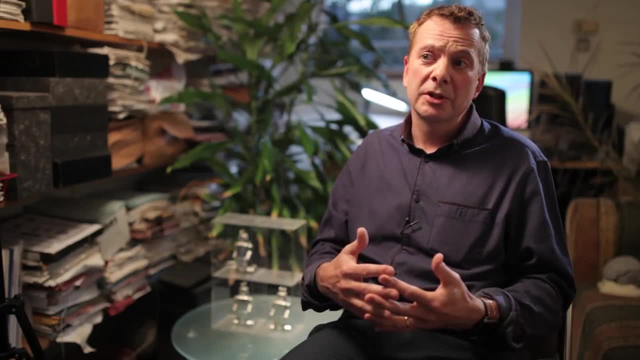 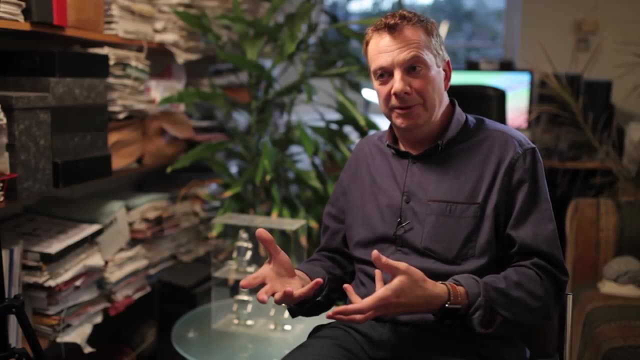 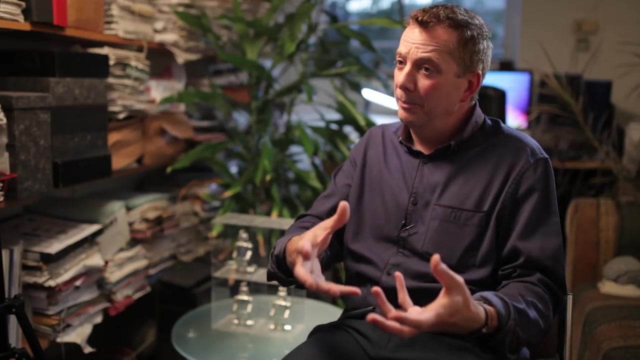 So you find a lot of these factors correlated with socioeconomic status. Which of those is having an effect on brain development and behavioral development? It's difficult to answer these questions, And neuroscience is using a set of different methods. We talked about brain imaging. 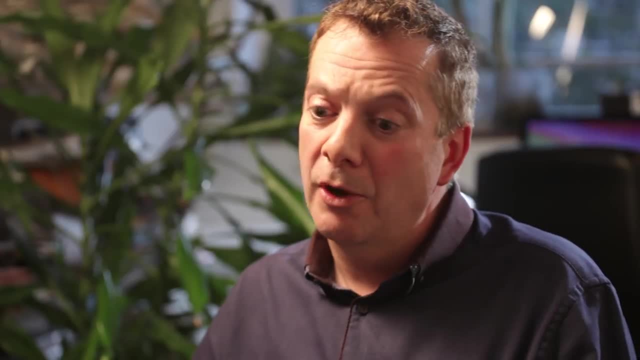 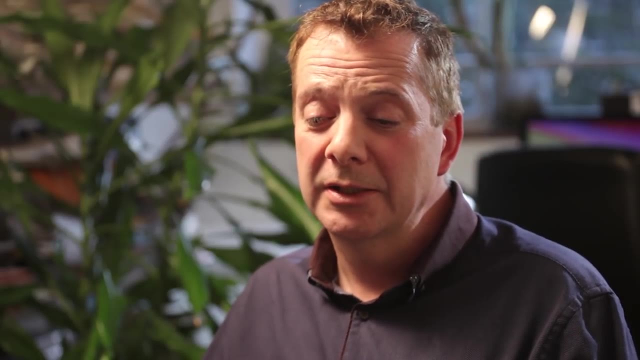 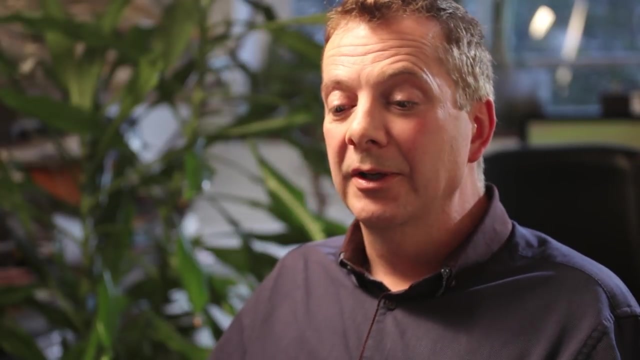 But also looking at animal models and computational models of the development of neural systems To try and understand the pathways by which this can take place. So typically we pull apart two different influences on families. We think about the level of stress in the family. 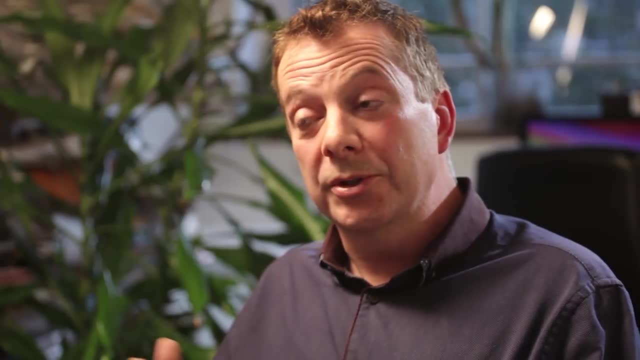 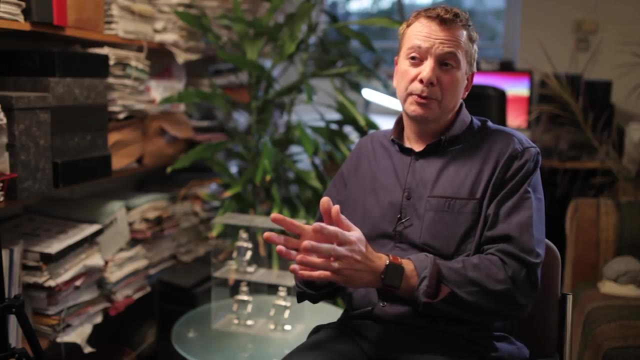 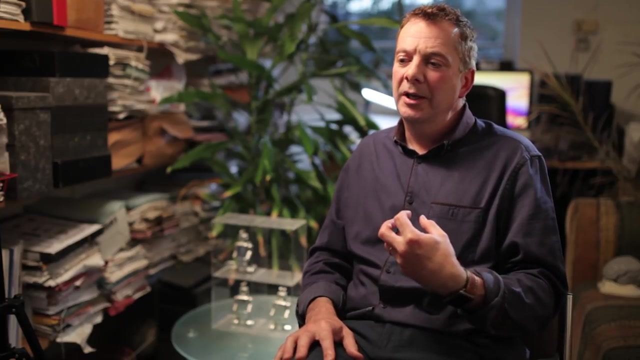 And these are kind of toxic effects of stress. We also think about the level of resources and opportunities in the family And then we map those into some possible causal pathways affecting brain development, And those are roughly of three different types. You can think of prenatal effects on a child's development. 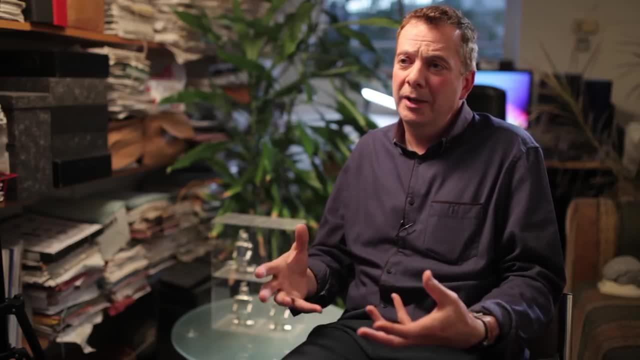 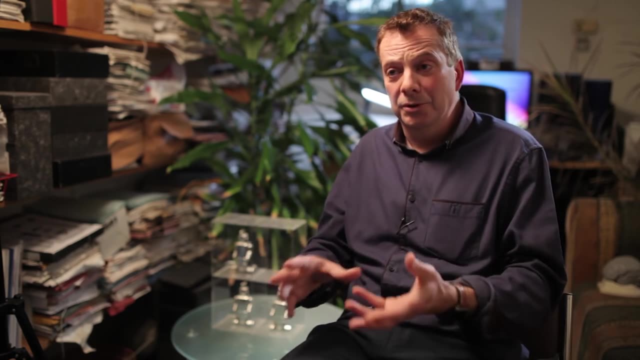 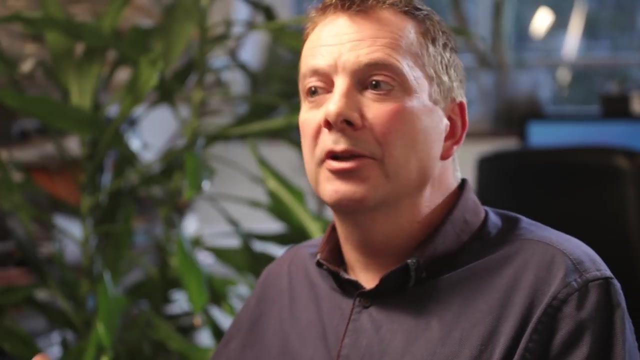 These are effects that will happen when the mother is pregnant. Maybe she's more stressed, Has poorer nutrition, Maybe she's more likely to smoke or drink. These are effects on the development of the embryo. The second type of effect would be postnatal parenting. 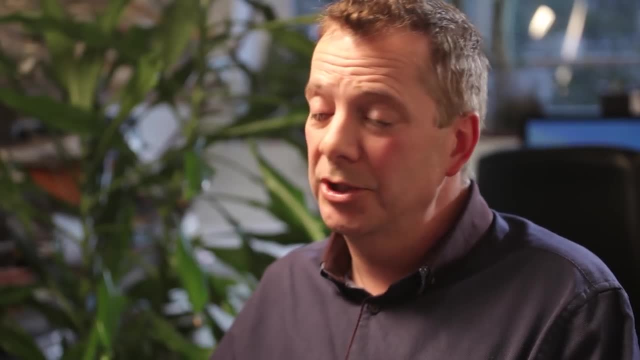 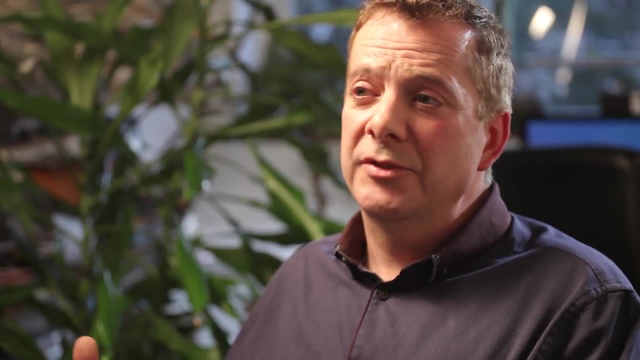 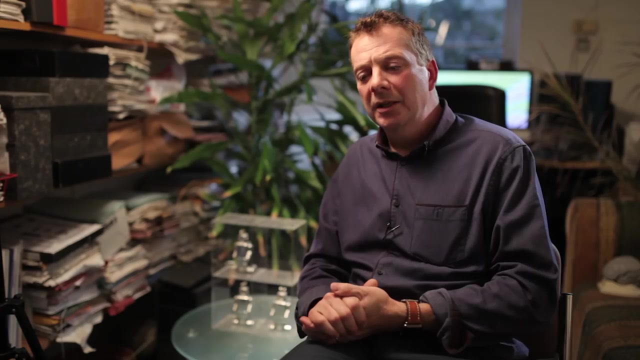 The nature of the relationship between the parent and the child And the nurturing that's happening. And then another type would be the level of cognitive stimulation, How rich the experiences are for the child. So these three different pathways, So we don't exactly know which of these. 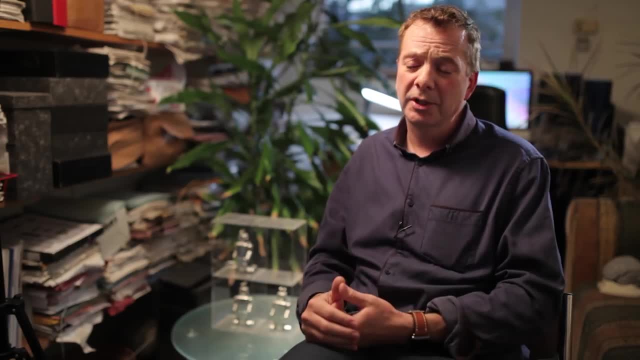 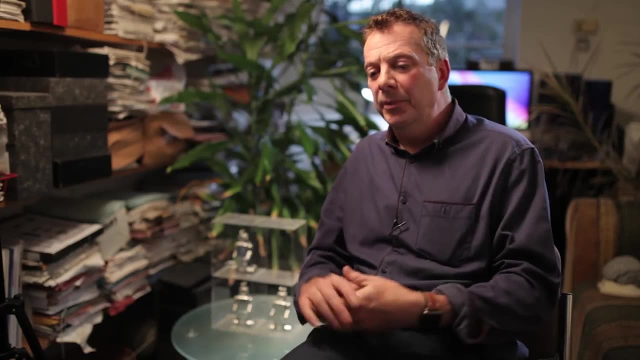 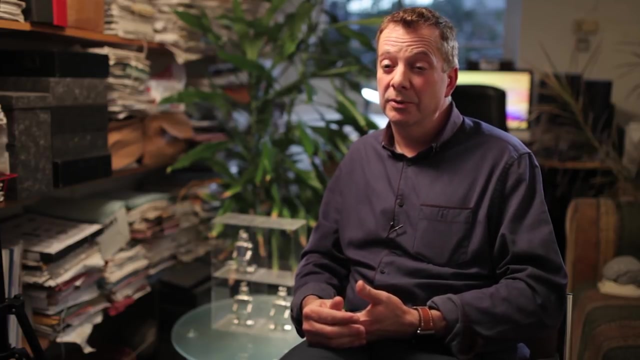 Are responsible And there might be different contributions of those causal pathways, Perhaps to different groups, Perhaps to rural poor versus urban poor. But here's one possibility about how it might work. We find slightly higher incidences of developmental disorders Like dyslexia and attention deficit hyperactivity disorder. 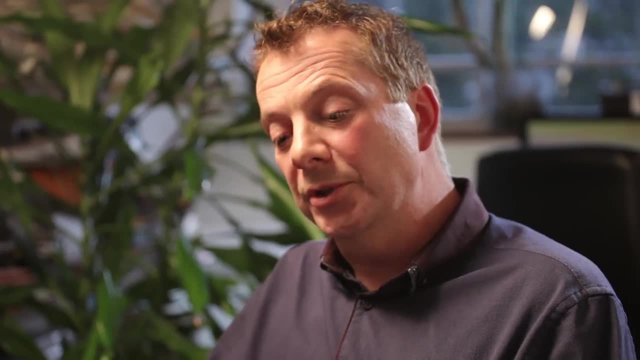 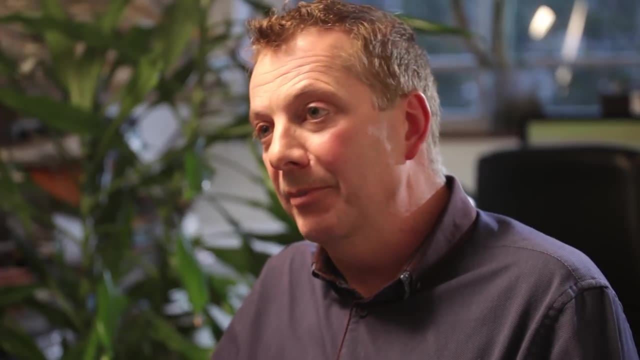 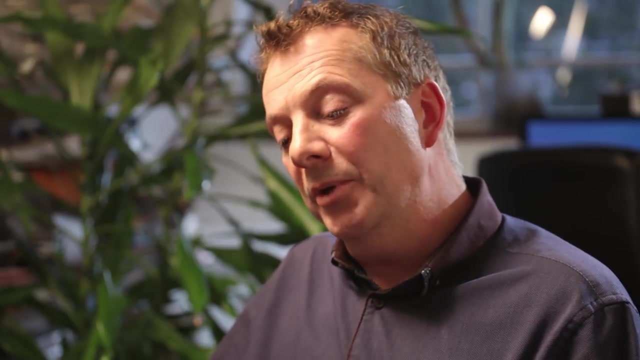 In children from poorer backgrounds. Maybe those are more to do with the prenatal effects, Where children have more behavioral problems And they can't regulate their emotions. Maybe that's coming more from the early parenting And the early nurturing, And maybe when we see differences in language development. 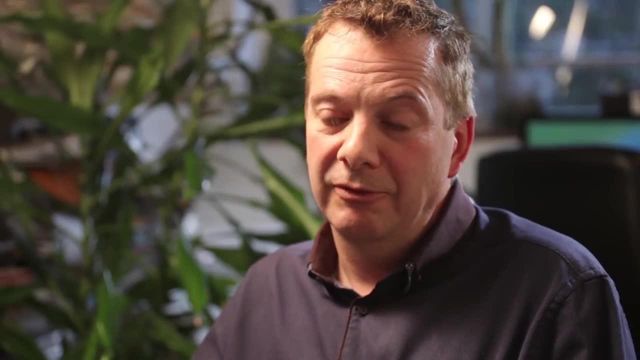 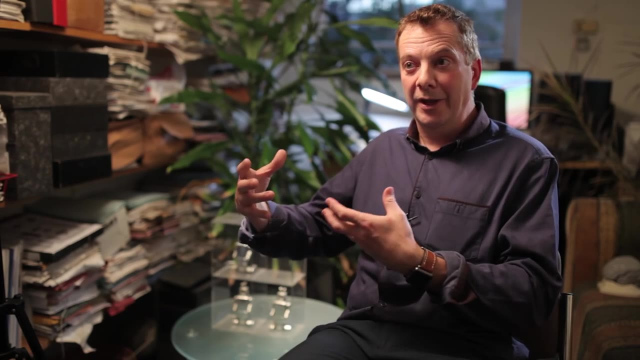 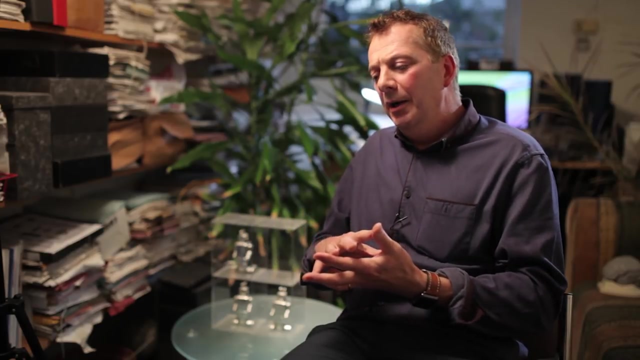 Maybe that's differences in stimulation in the environment And then maybe children's just natural experience in the physical world Is enough to allow their spatial skills to develop Sort of independently from their socioeconomic status. So In this study of socioeconomic status from a cognitive neuroscience perspective,